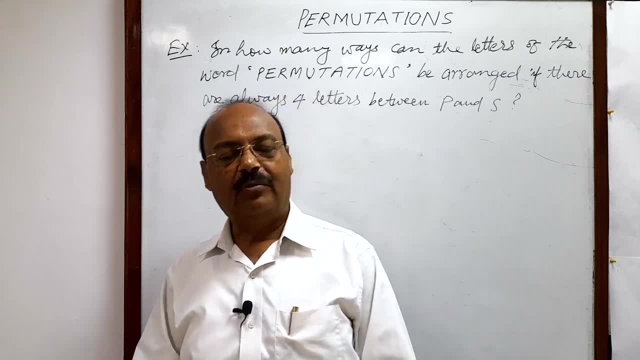 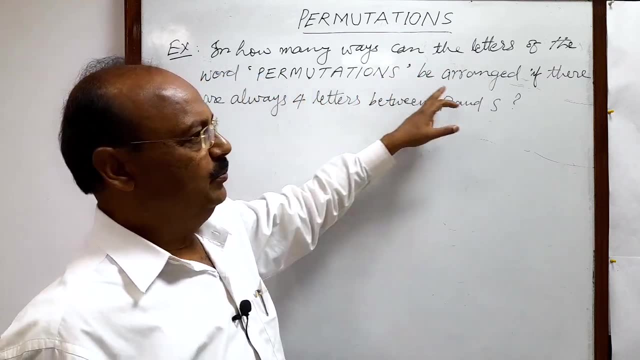 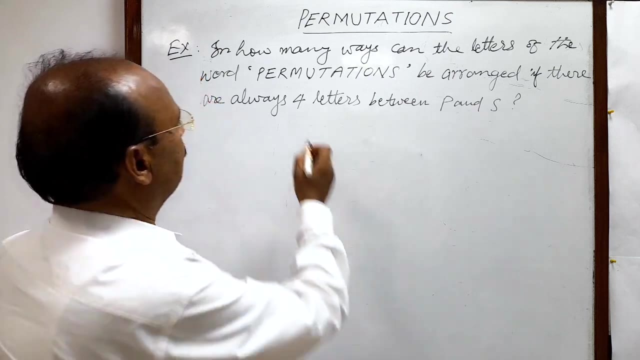 Welcome students. Here we will see a very interesting question from the chapter permutations. Here question is: in how many ways can the letters of the word permutations be arranged if there are always four letters between P and S? So this word is given permutations. given word is permutations. 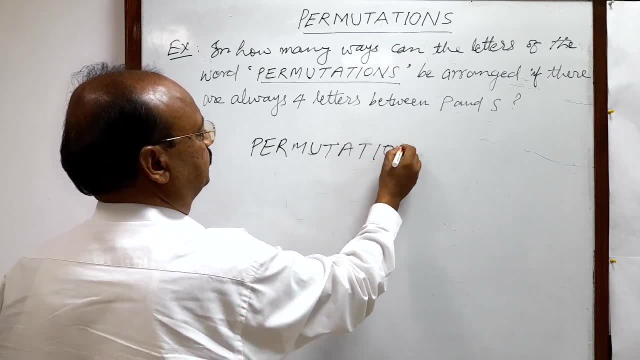 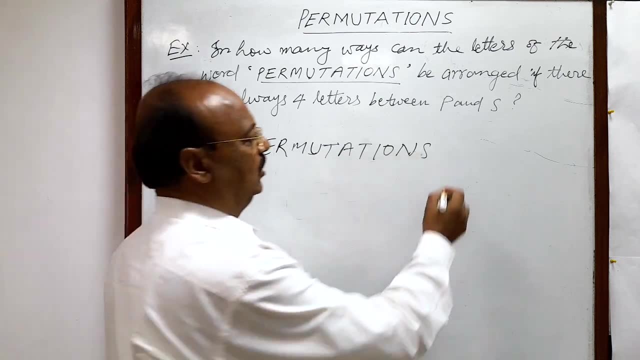 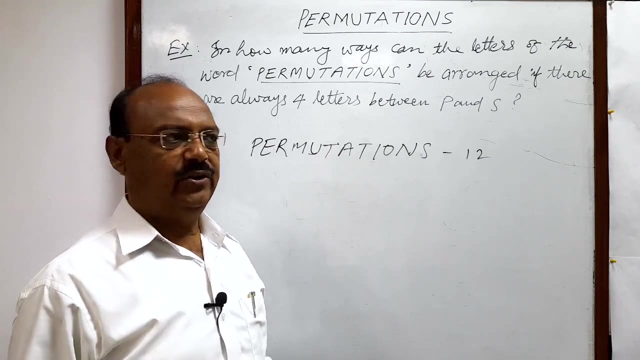 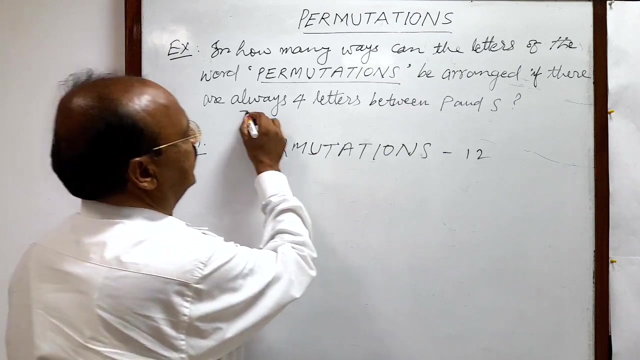 Here, total number of letters is 1, 2,, 3,, 4,, 5,, 6,, 7,, 8,, 9,, 10,, 11, 12.. Okay, so there are 12 letters here And with the help of these 12 letters, we have to make different arrangements on total number of words with or without meaning, considering the condition that there are always four letters between P and S. 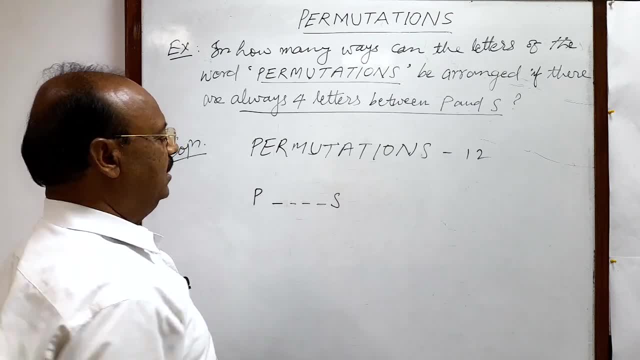 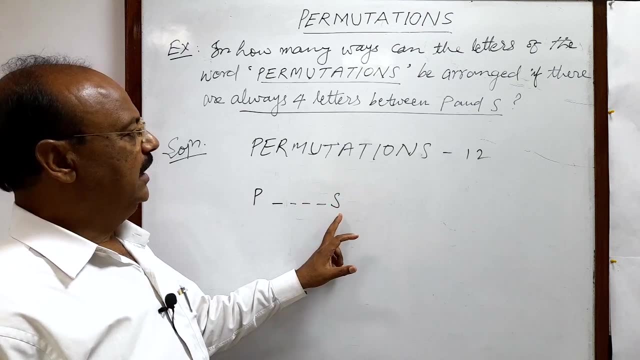 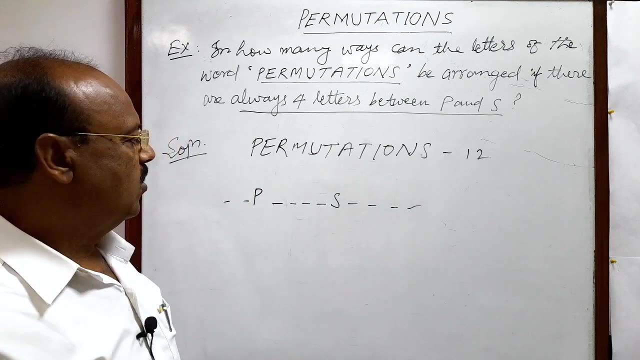 So P and S, in between P and S, there should be always four letters. So these four letters and 5 and 6 and remaining 6 letters will be either this side or this side, like this. Okay, so we have to find out the number of arrangements. 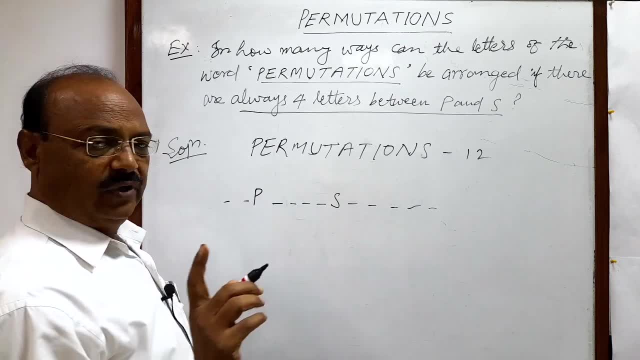 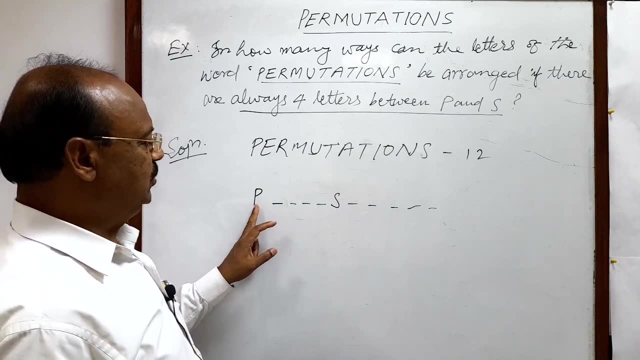 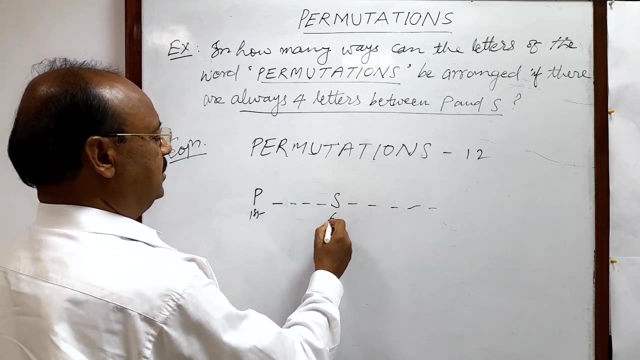 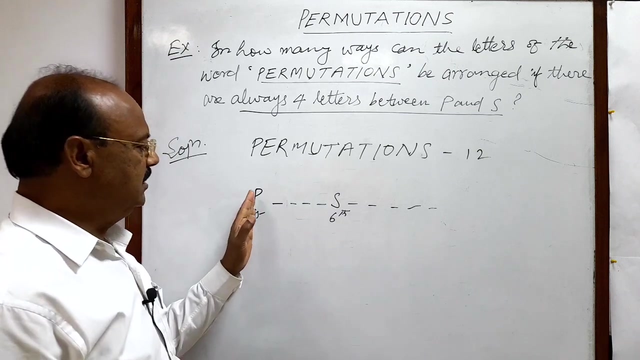 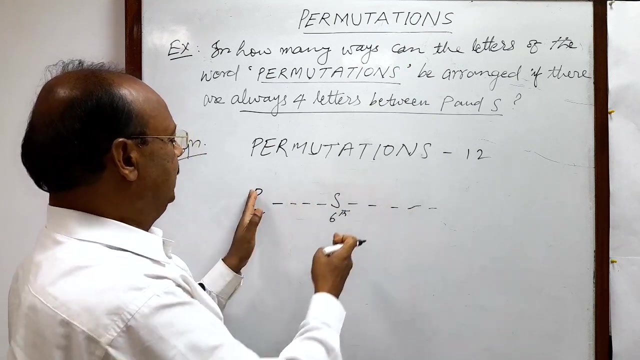 Now suppose we consider this arrangement where P is between P and S. So P starts from the first position, P is in first position and S will be in sixth position, Isn't it? This is in first position and this is in sixth position because in between there are four letters. So this is one option. But this point, this number, this letter, P and S may shift from here. There is no problem. P may come here, P may come here, P may come here. Accordingly, S will shift. 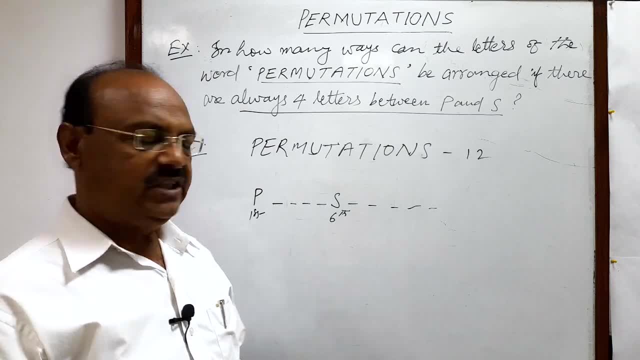 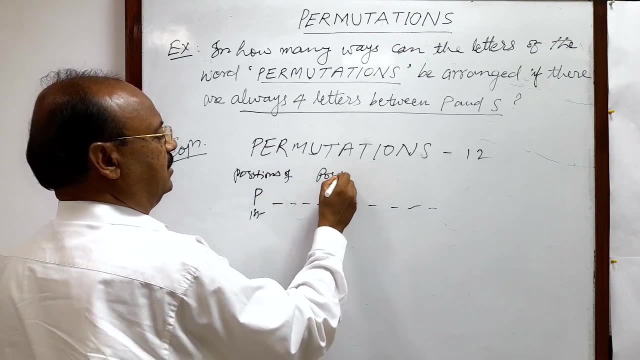 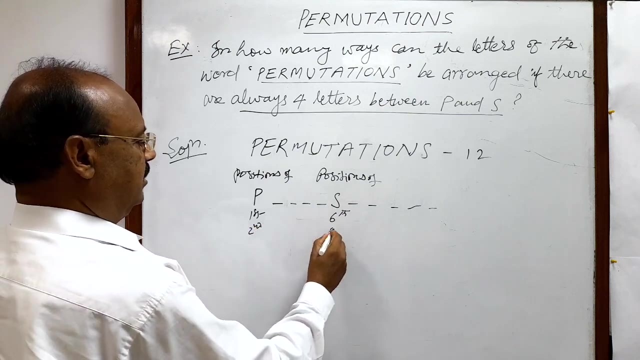 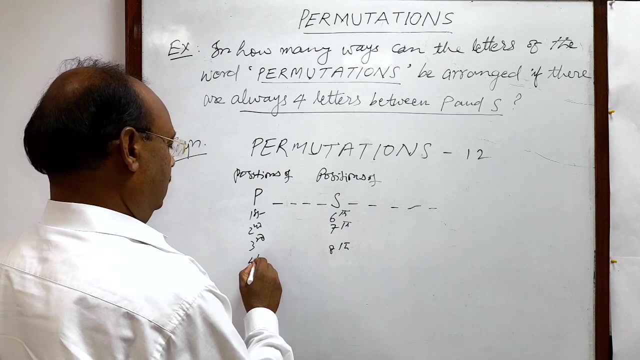 So, first of all, we will try to understand what are the different positions, different positions of P and different positions of S. One position is first and sixth, Another is second, and this is third and eighth, fourth and ninth, fifth and seventh. 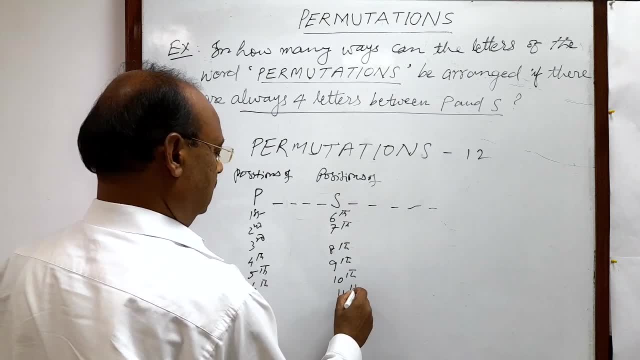 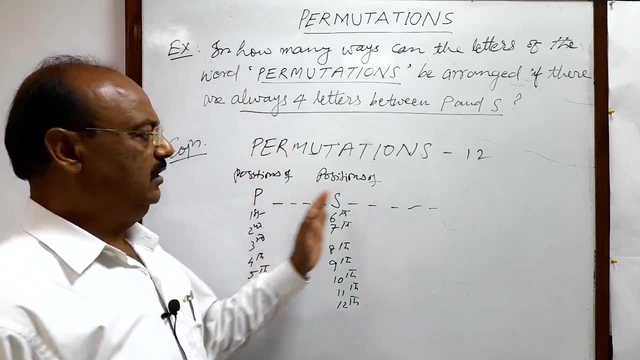 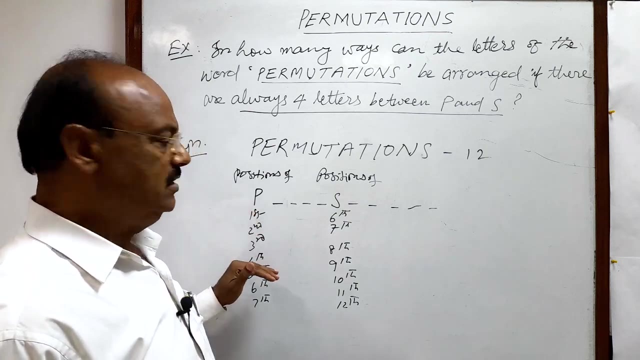 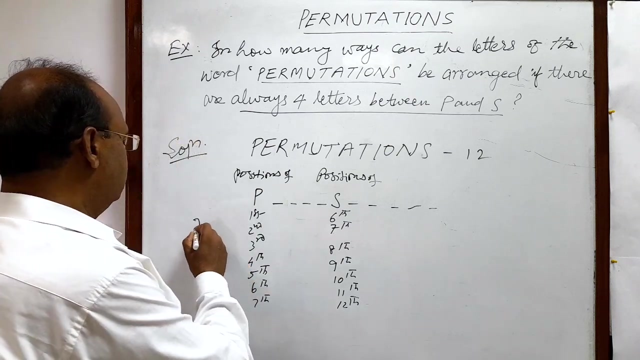 And sixth and tenth, sixth and eleventh, seventh and twelfth, Because there are only twelve letters, So we cannot exceed this twelfth position. Okay, So there are how many different positions of P? How many different options for P and S? In total there are seven options. So these seven options we have here, Okay, 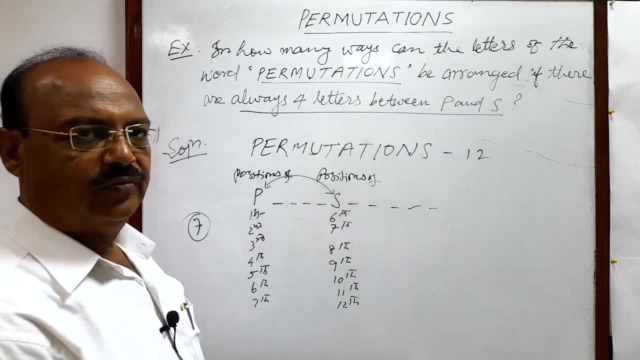 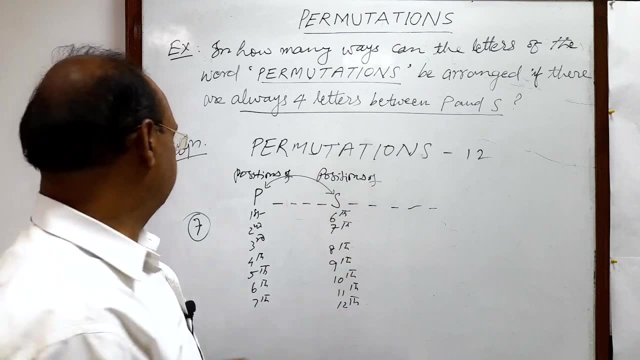 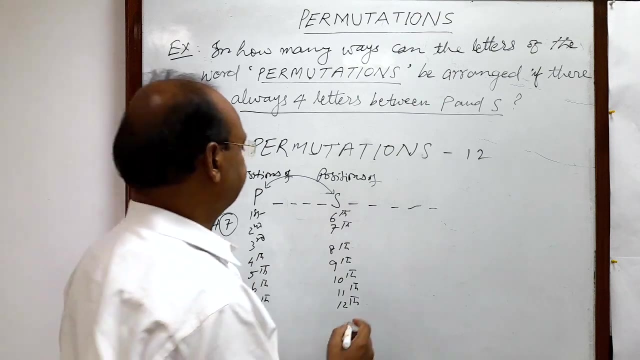 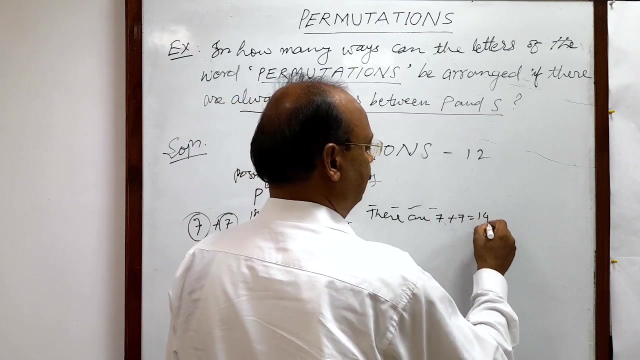 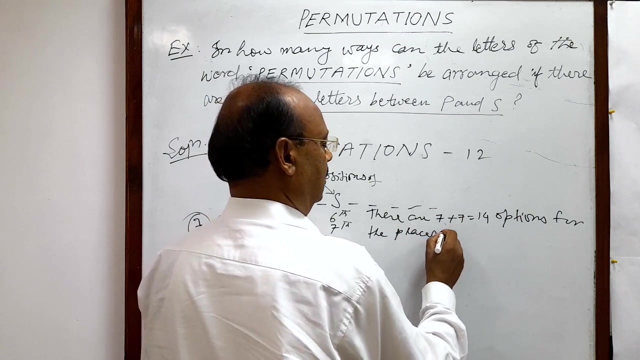 Now these two letters can interchange their places, so another seven options we will have when s will be here and p will be where, then other seven options will be. so 7 plus 7 is equal to: there are 14 options. okay, so here we can write: there are: 7 plus 7 is equal to 14 options for the places of p and s. 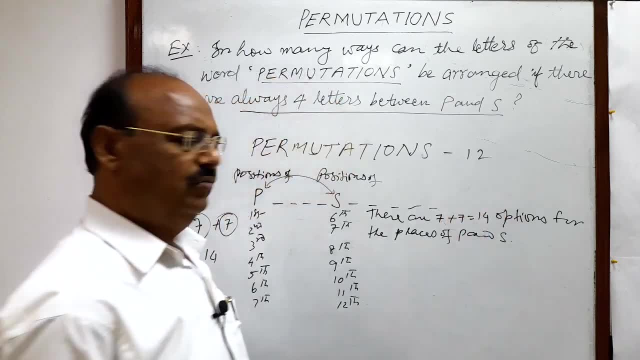 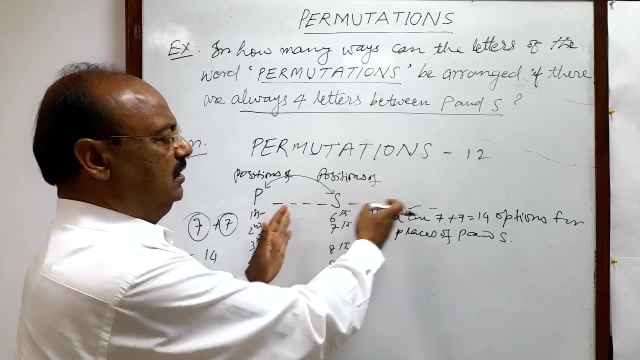 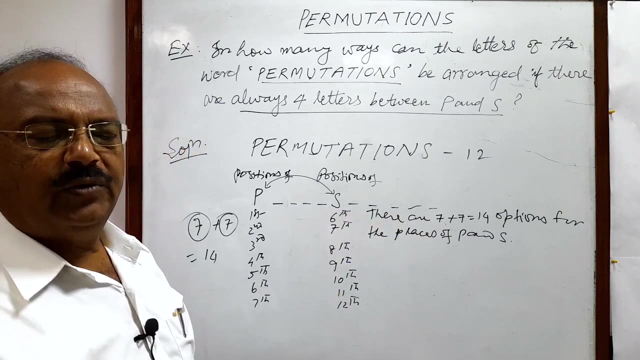 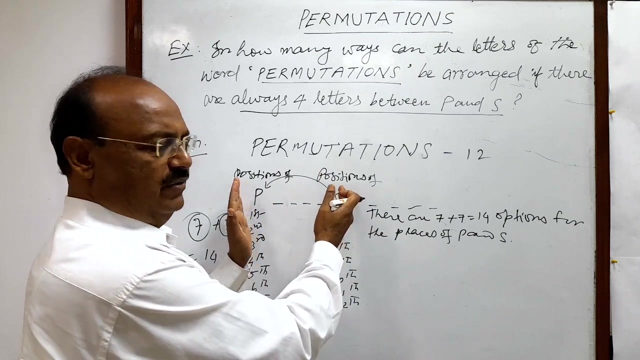 okay. so we have to fix p and s and rest. 10 letters may lie anywhere suitably okay. so we have to fix p and s and rest 10 letters may lie anywhere suitably okay. So under the consideration of number of permutations, number of arrangements will take P and S because for any certain condition they are fixed in fixed place. So only there will be arrangements of other 10 letters. In how many ways? 10 factorial ways. 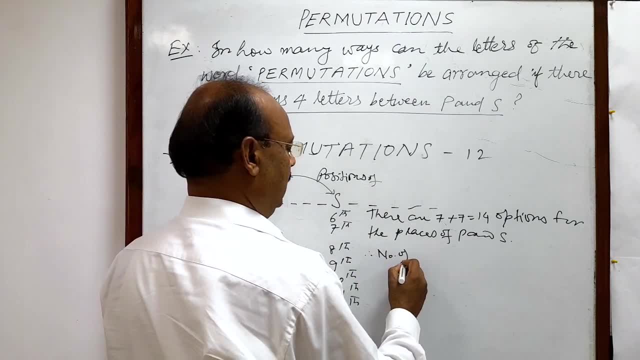 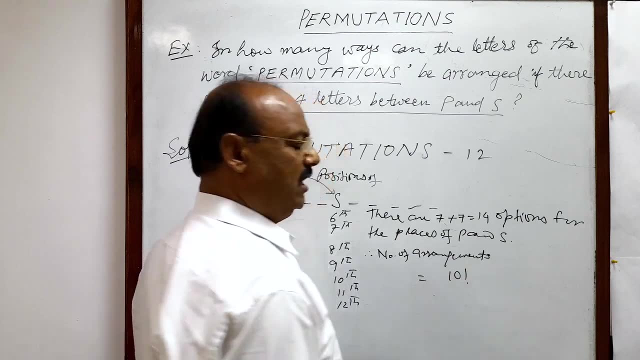 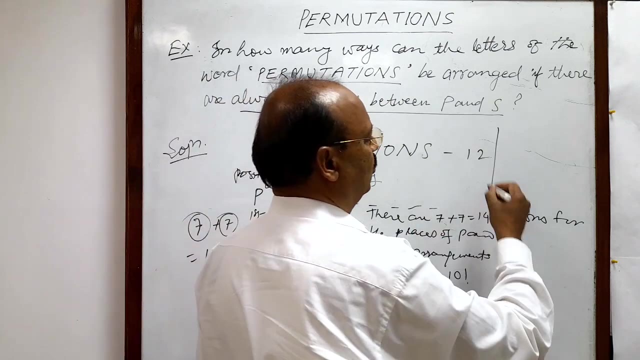 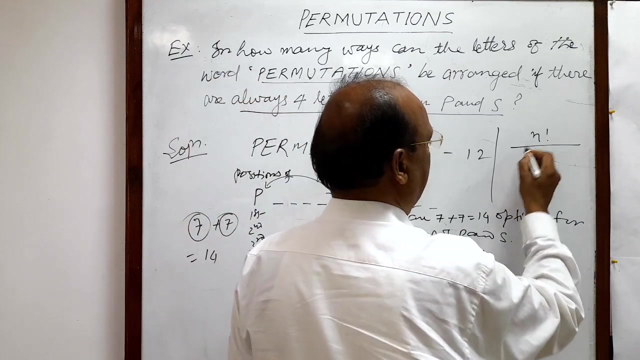 So therefore, number of arrangements will be 10 factorial ways, And in several questions, several times, we have discussed that in this chapter- there is a formula that when all the objects are not different, some of the objects are alike. then there is a formula of arrangements- N- factorial, by P, factorial, Q factorial, R- factorial, like this: 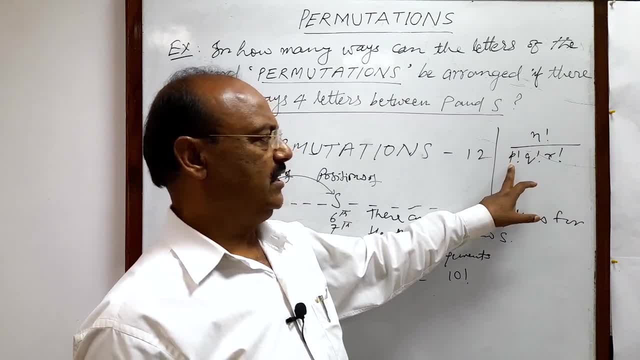 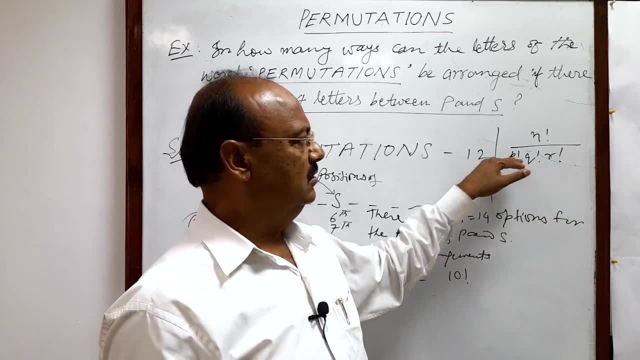 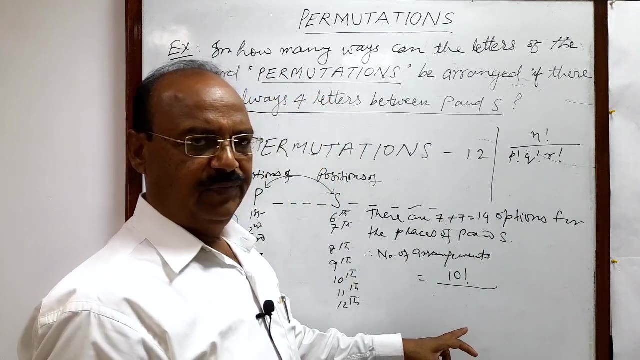 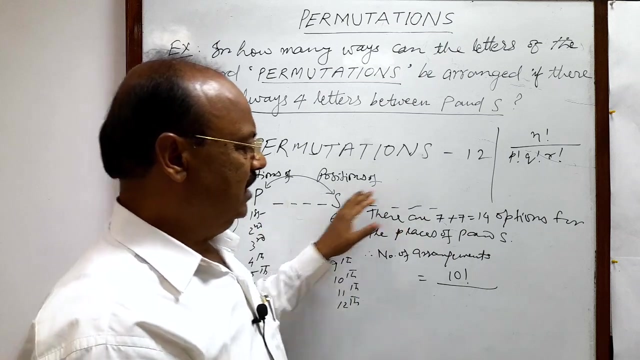 If N is the total number of objects And P objects are alike of one kind, Q objects are alike of another kind, R objects are alike of another kind, then we will write this formula: So, similarly here, total number of objects is 10 here. So this will be 10 factorial. As we have discussed, P and S are fixed for particular case, So there will be no chance of arrangement of P and S. Rest of the 10 letters will arrange among themselves. So this is 10, factorial, Correct.